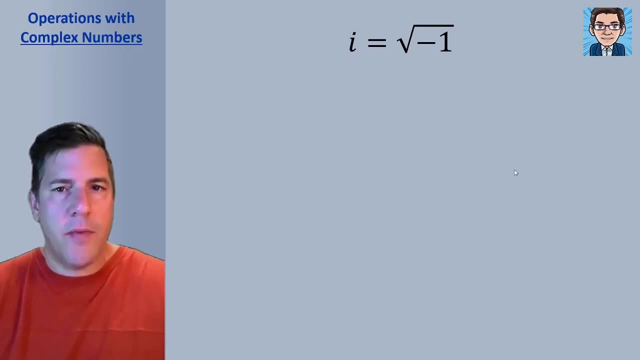 Now, an important concept when you're doing operations with complex numbers is I squared. So if I is the square root of negative 1, then I squared is going to be the square root of negative 1 times the square root of negative 1,, which just ends up being negative 1.. 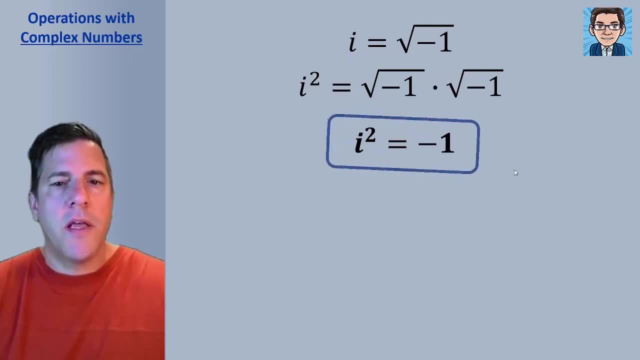 So a very important concept when we're doing operations with complex numbers is that I squared is negative 1.. So whenever we're doing operations, we treat a variable i just the same as any other variable. So if we had 5i plus 10i, we would get 15i. 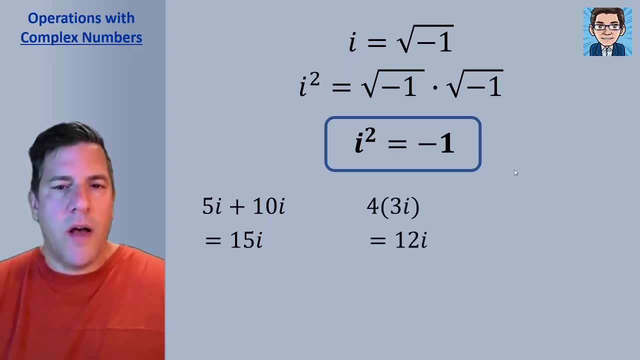 4 times 3i, we would get 12i. But when we get a case like this, 6i times 5i, we'd get 30i squared. But rather than a regular variable, we've got to go one more step now. 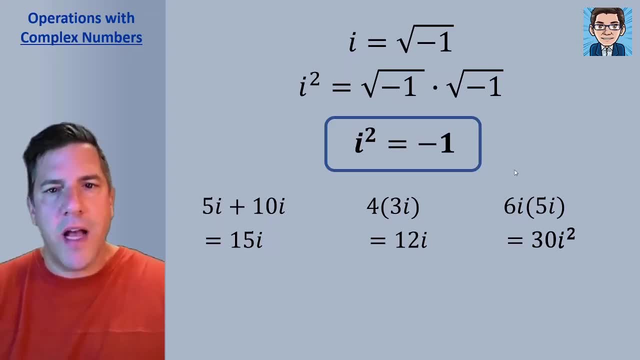 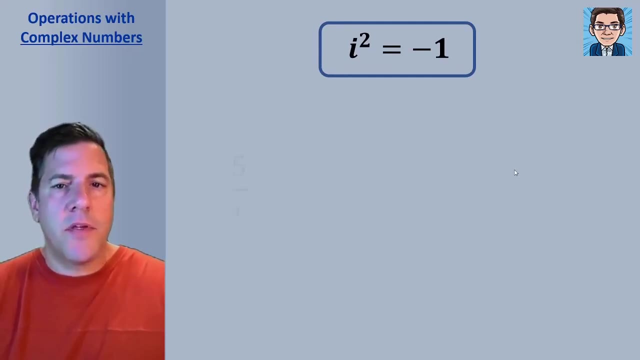 because the i squared is equal to negative 1, so we've got to replace the i squared with negative 1.. And this becomes 30 times negative 1, or just negative 30.. Okay, let's take a look at how to simplify something. 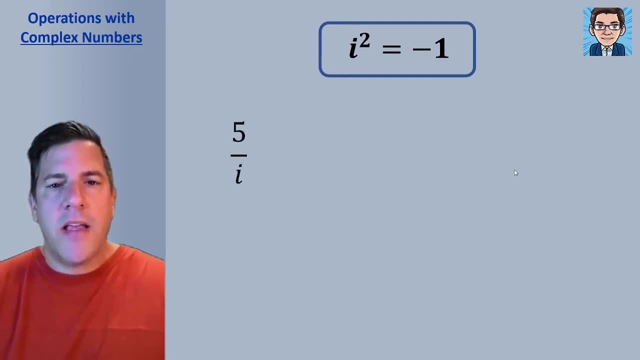 So if we have i in the denominator, since i is defined as a square root, we can't have a square root in a denominator to have something fully simplified. So 5 over i, we can simplify that by multiplying. We're multiplying both the numerator and denominator by i. 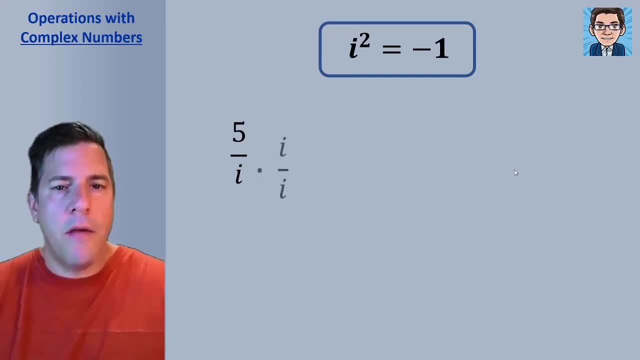 So if we multiply the numerator and denominator by i, we're multiplying by 1, so we can do that. So the numerator is going to be 5i and the denominator is going to be i squared. And again we need to know that i squared is negative 1, and we're going to replace i squared with negative 1.. 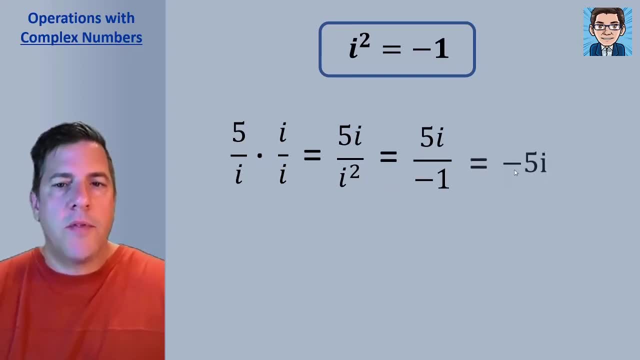 So then 5i over negative 1 just becomes negative 5i. Okay, So if we have a more complicated, where we've got that was just an imaginary number in the denominator- what if we have a complex number in the denominator? 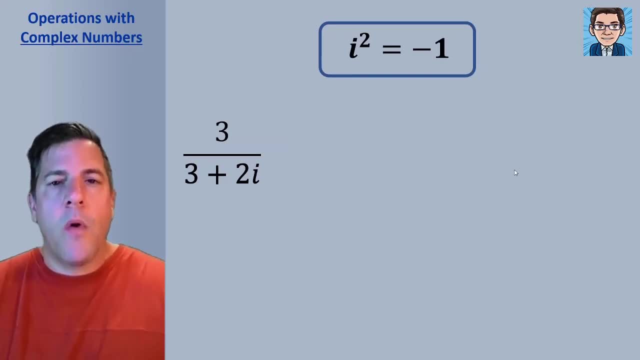 How would we simplify 3 plus 2i? Well, we're going to multiply it by something that's called the conjugate. So the conjugate of 3 plus 2i is going to be 3 minus 2i, And you'll see why we chose that particular thing in a second. 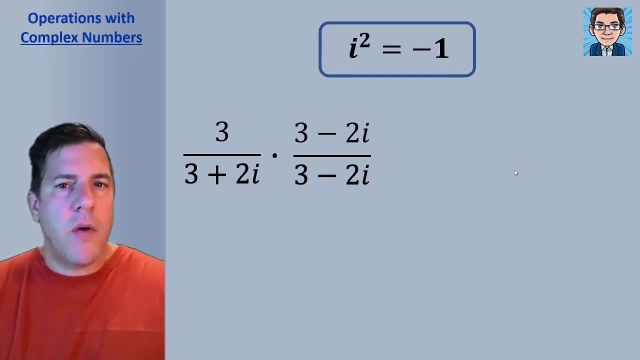 And it's just because that's going to help us cancel out, so we have no more imaginary number in the denominator. Let's see how that's going to work. So if we multiply the numerator The 3 times the 3 is 9, and the 3 times the minus 2i is going to be minus 6i. 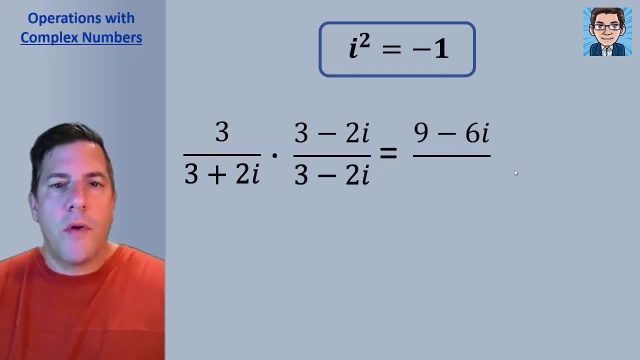 But let's take a look at what we do with the denominator. So the denominator: we've got to multiply 3 plus 2i and 3 minus 2i. So let's multiply this out by FOIL. The first 2 is going to get us 9.. 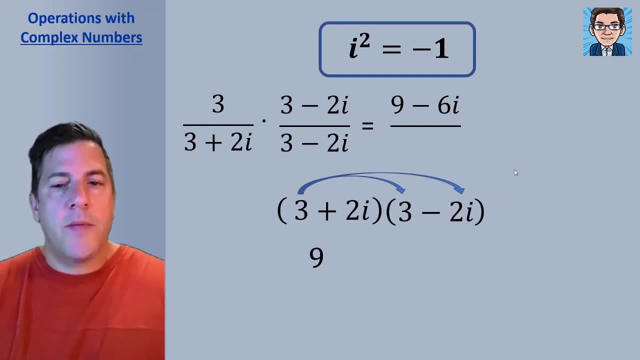 The last 2, I mean the outers- is 3 times the minus. 2 is going to get us minus 6i. The inners, the 2i and the 3. It's going to get us plus 6i. 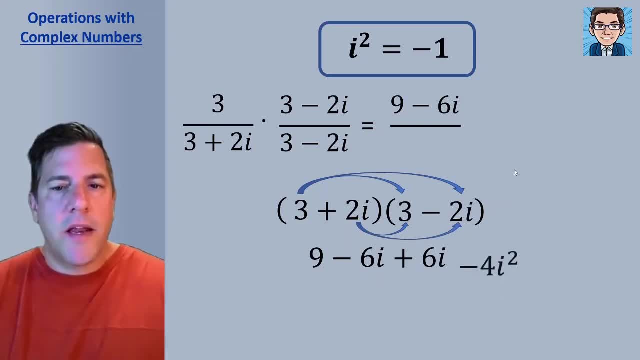 And the last 2, the 2i and the minus 2i is going to get us minus 4i squared. Now, when we do the math here, the minus 6i and the plus 6i cancel out, And those middle 2 terms are always going to cancel out when we pick a conjugate. 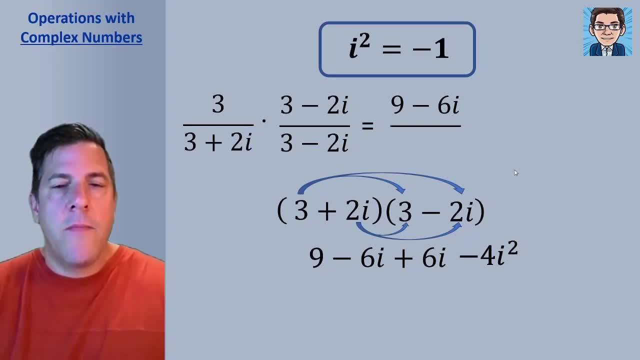 When we pick the same 2 terms but a different sign, those 2 middle terms are going to be the same, except with different signs, and they're going to cancel out. So those 2 are going to cancel out. We're just going to be left with 9 minus 4i squared. 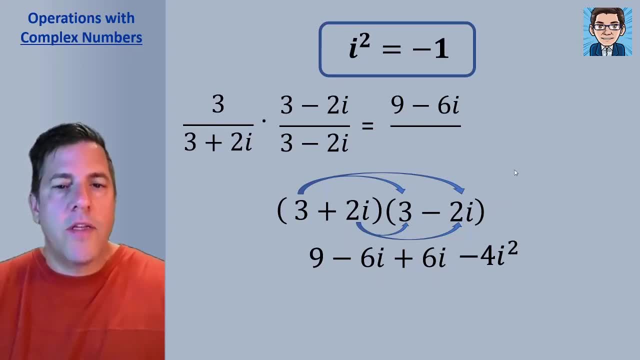 But we're going to replace that i squared with negative 1.. So this becomes 9 minus 4 times negative 1, or 9 plus 4 or 13.. So that whole denominator now has no imaginary number in it anymore, So it's just a whole number. 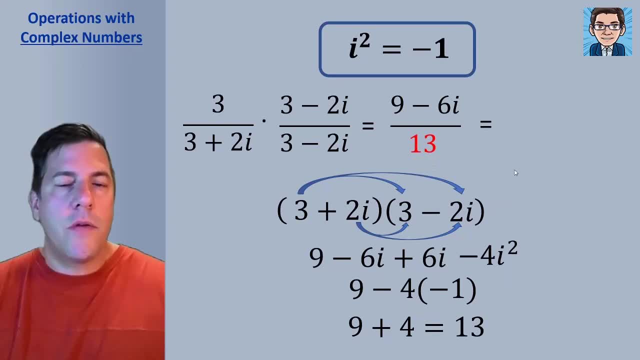 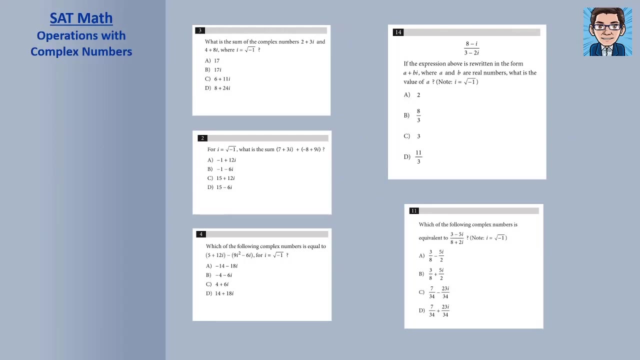 So that denominator is 13.. And then to do the final step, to simplify this, we just split it up into 2 parts: The 9 over 13 and the minus 6 over 13i. Okay, I've got 5 problems picked out from the official practice SAT test. 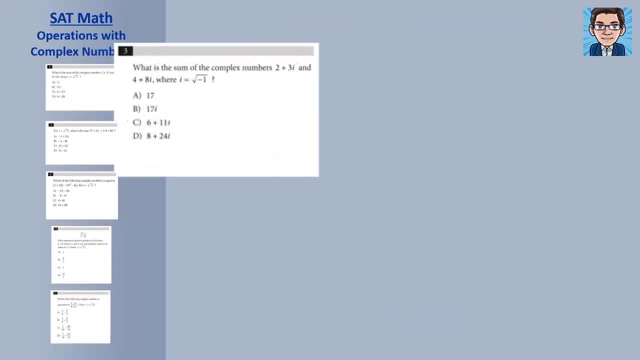 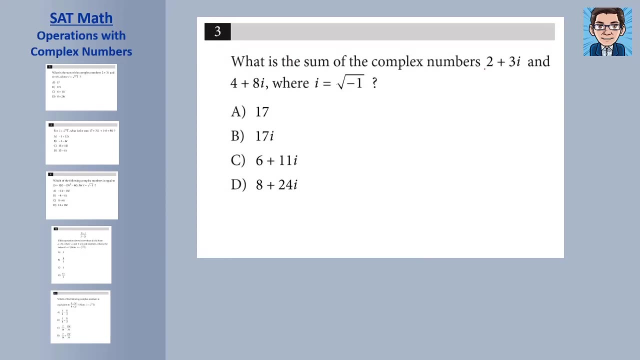 Let's take a look at these. First one, very straight forward, We've got 2 plus 3i and 4 plus 8i. We're just going to combine our like terms. We're going to combine the real part. 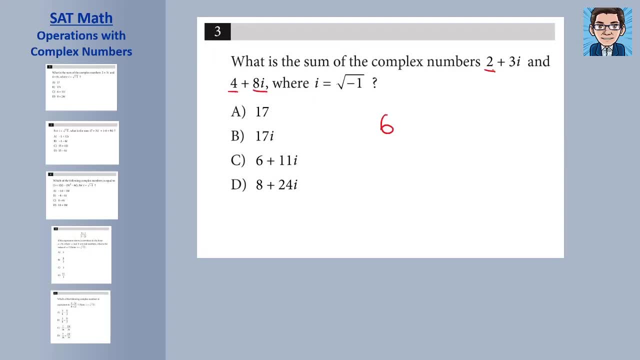 The 2 and 4 is going to get us 6. And then just combine the imaginary part 3i and 8i and we get 11i, And we really don't have to go any further from that, And c is our answer. 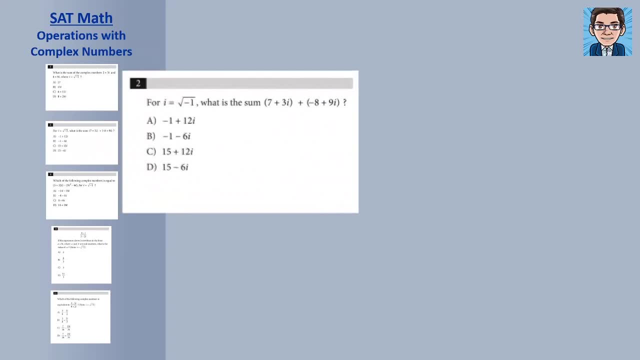 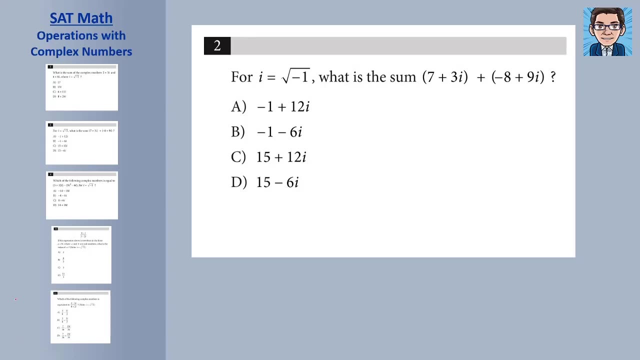 The second one very similar. Let's combine our like terms. So if we combine the 7 and the minus 8, we're going to get negative 1.. The 3i and 9i is going to get us 12i. 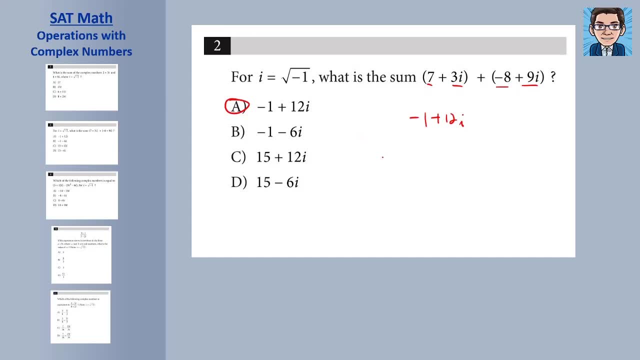 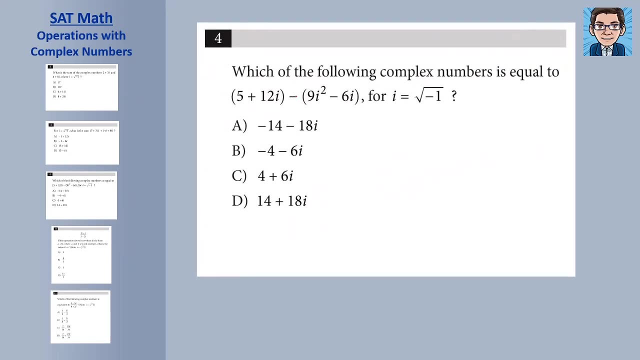 And then that gets us choice a. The third problem gets a little trickier. We're subtracting And we also have this i squared in here. The best thing to do first is to get rid of that i squared. The key important thing is to remember the i squared is negative 1.. 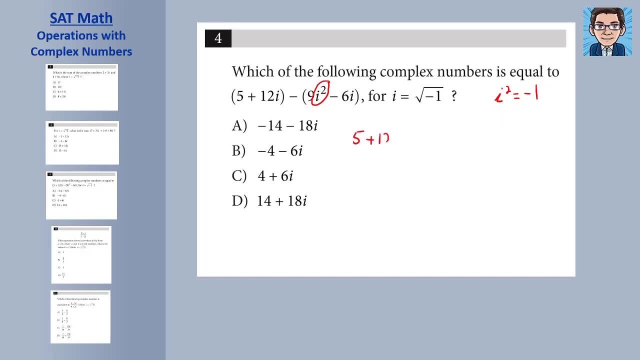 So let's rewrite this Now: the 9 times i squared i squared is negative 1.. So 9 times negative 1. Is going to get us negative 1. Negative 9 here. Then we've got to be careful when we're subtracting. 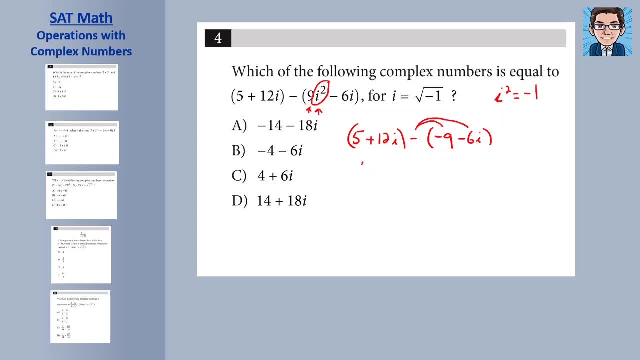 We've got to subtract both pieces, So this is going to be 5 plus 12i. minus a negative 9 becomes a plus 9.. And then minus a negative 6i becomes a plus 6i. Then from there we just combine our like terms. 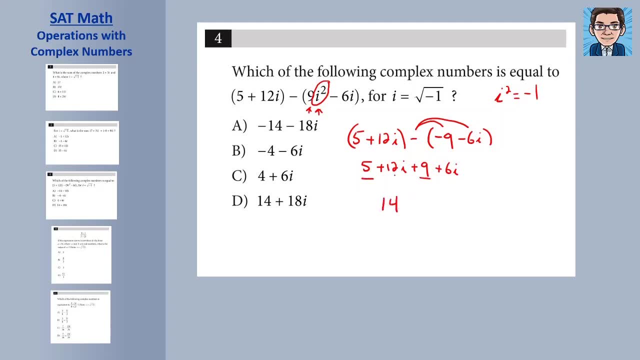 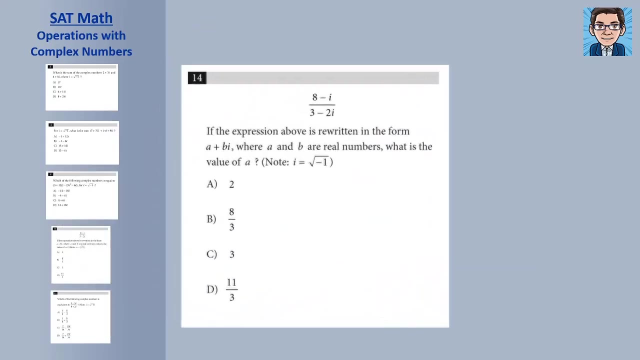 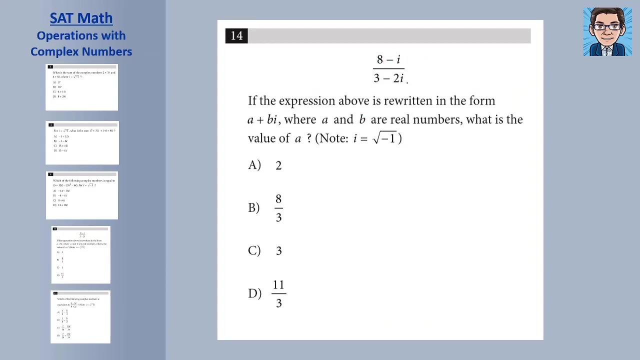 5 and 9 is going to be 14.. The 12i and 6i combine to 18i, Which matches our answer d. Okay, Here we're dividing two complex numbers: 8 minus i and 3 minus 2i. 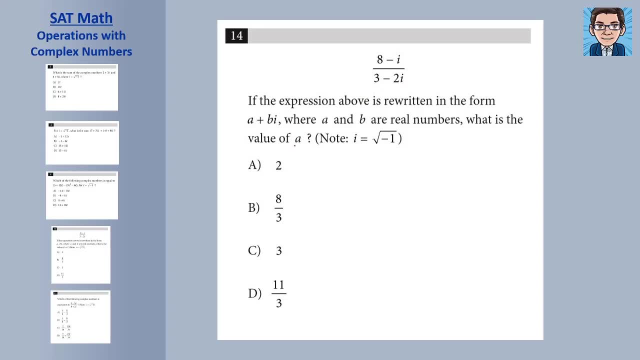 But notice what they're looking for. They're only looking for the real part. So they're only looking for a, The real part of the complex number. So we're still going to have to multiply this by the conjugate. So we're going to multiply the denominator. 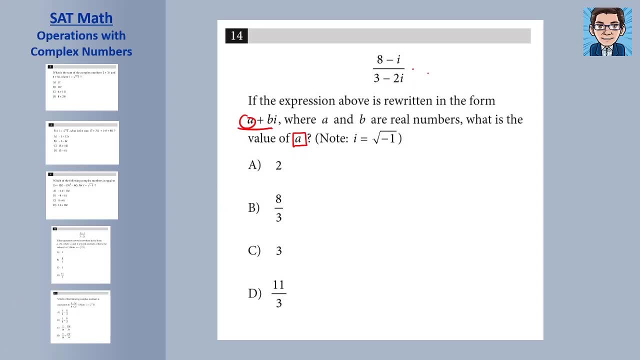 By 3 plus 2i. And then we also have to multiply the numerator by 3 plus 2i. Alright, So now let's calculate what the numerator is going to be. The numerator is going to be 24.. Now here's a little shortcut. 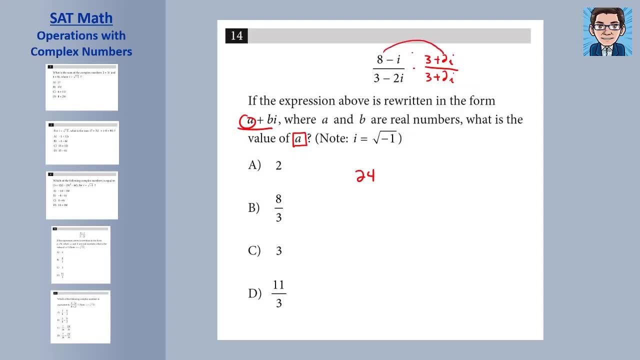 You can multiply it all out if you want, But this term and this term are going to be imaginary numbers, So we actually don't need those. We're going to have plus something times i, And then our last term is going to be minus 2i squared. 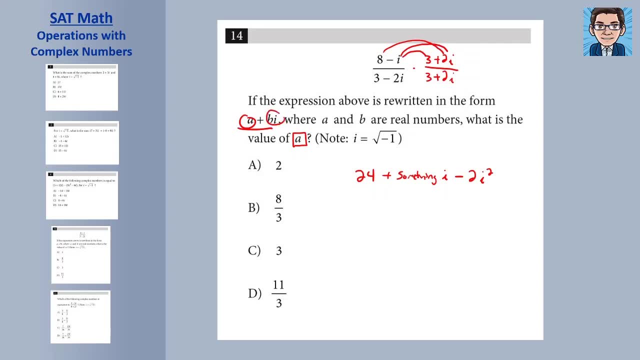 And if you wanted to calculate those, you can, But that's going to get us the b part And then, so you're just going to get for the numerator, You're going to get 24 plus 2.. Because the i squared we're going to replace with negative 1.. 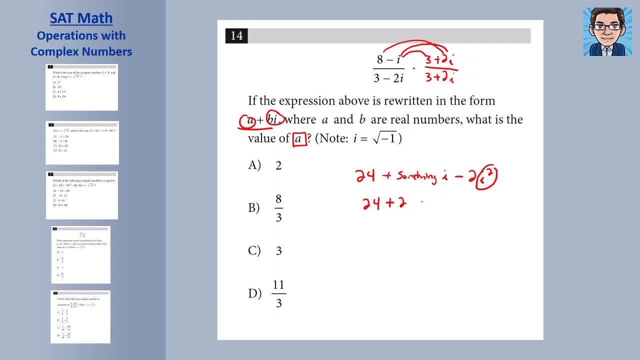 Negative 2 times negative, 1 is going to be plus 2.. So the real part of the numerator is going to be 26.. So this is going to be 26 plus something i, Alright, And then the denominator, The 3 minus 2i and the 3 plus 2i. 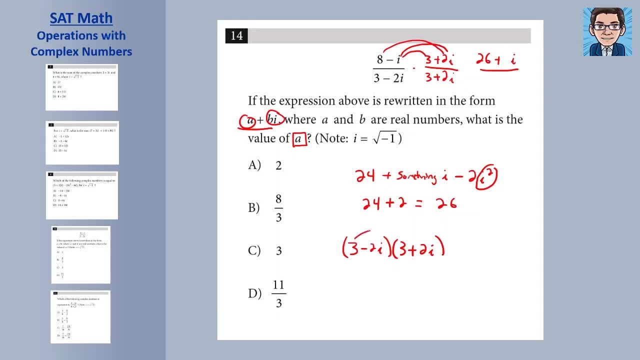 When we multiply conjugates, our middle terms are going to cancel out, So we're going to get 9.. We're going to get a plus 6i and minus 6i. They cancel each other out. And then we're going to get a minus 4i squared. 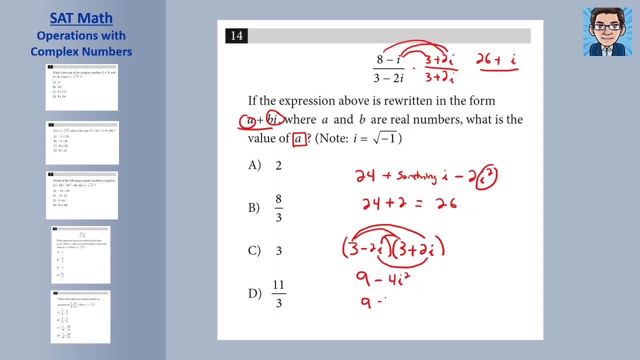 We replace our i squared with negative 1. And we get 9 plus 4 or 13. So our denominator is going to be 13.. So our real part, the a that we're looking for, is going to be 26 over 13 or 2.. 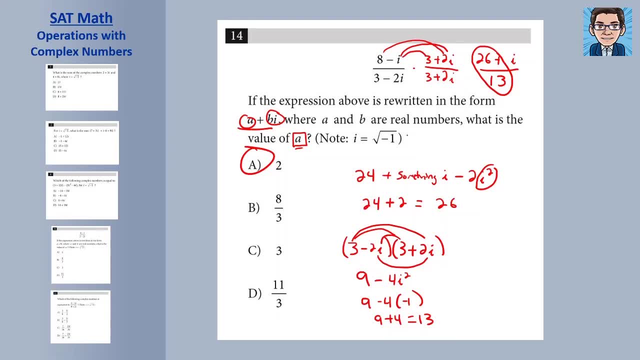 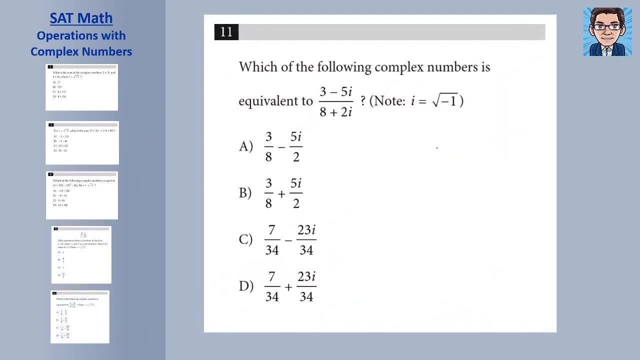 And again, if they were looking for the full answer, we would just have to calculate these, And then we would have an i as well. Alright, Here we're dividing two complex numbers. We're going to have to multiply by the conjugate. 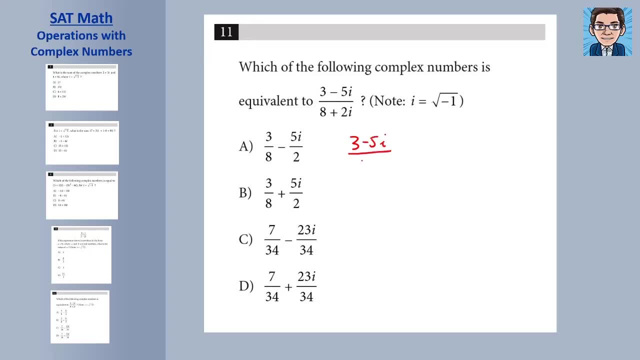 So we're going to have to multiply 3 minus 5i over 8 plus 2i. The conjugate of the denominator same terms with a different sign is going to be 8 minus 2i. Multiply the top of the numerator and denominator both by 8 minus 2i. 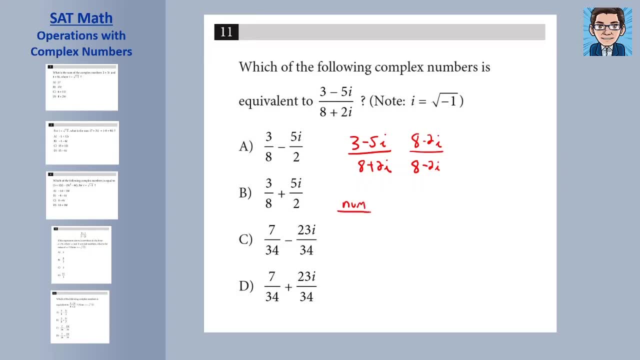 So let's do it out. The numerator is going to be: Let's put parentheses around these just to make it a little easier to see. We're going to get 24, the 3 times the 8. We're going to get minus 6i, minus 40i. 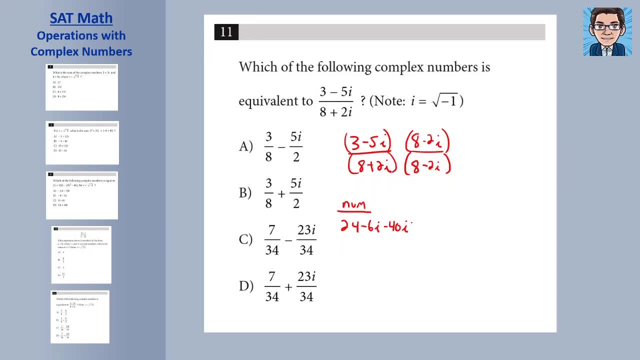 And then plus 10i squared, Minus 5i times minus 2i is going to be plus 10i squared. Now we're going to combine our like terms. That's going to get us minus 46i. And then, since these are complex numbers, i squared is negative 1.. 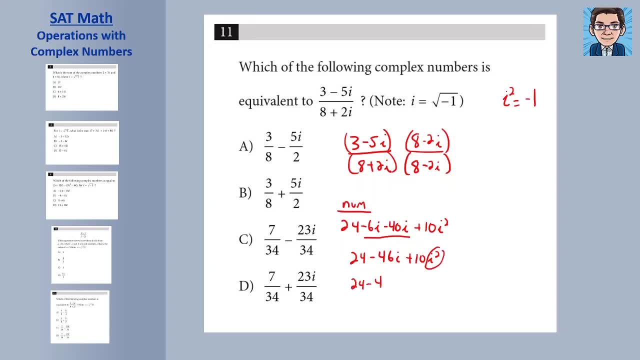 So we're going to replace this i squared with negative 1.. 24 minus 46i, plus 10 times negative 1. Or minus 10.. So when we combine the 24 and the minus 10, we're going to get 14 minus 46i. 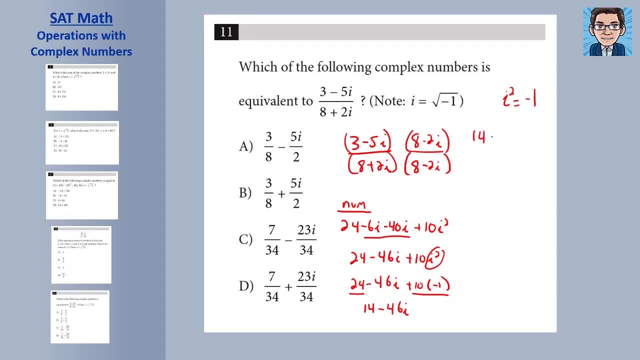 So that's our numerator. It's 14 minus 46i. Now let's work on the denominator. So our denominator- The middle terms are going to cancel out, So we're just going to get 64.. 8 times 8 is 64.. 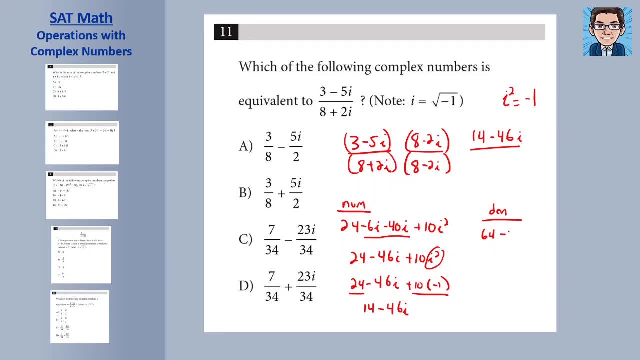 2i and minus 2i is going to be a minus 4i squared. We're going to replace that i squared with a negative 1.. And we can get 64 plus 4. Or 68.. 68.. Then we divide this up into two parts. 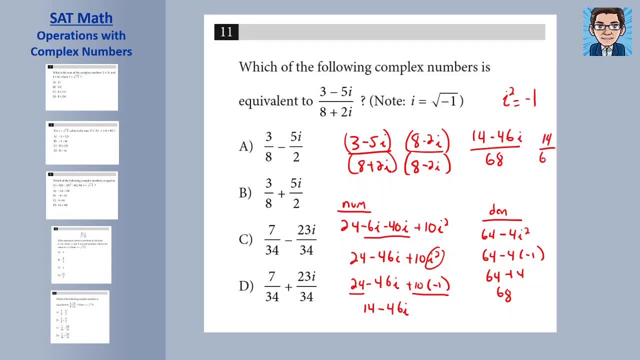 We're going to get 14 over 68 minus 46 over 68i, And we can just reduce both of those fractions. Divide everything by 2. We're going to get 7 over 34. And 23. And it's a minus. 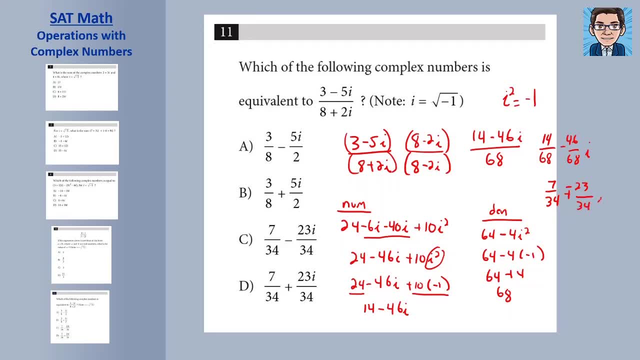 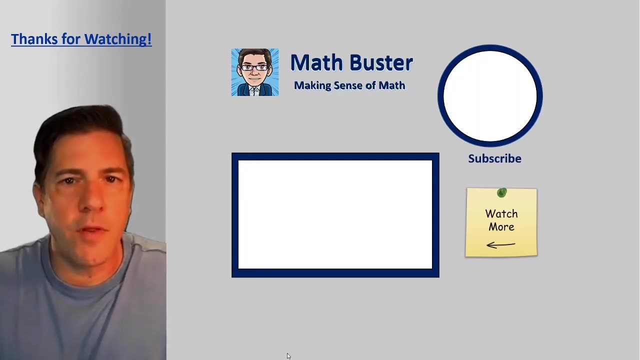 23 over 34.. 3 over 34i And that's going to match our answer C. Thanks for watching And if you have an SAT coming up, good luck. I'm going to continue to add SAT material. So if you'd like to subscribe right up here, you can get notification of when new material comes out. 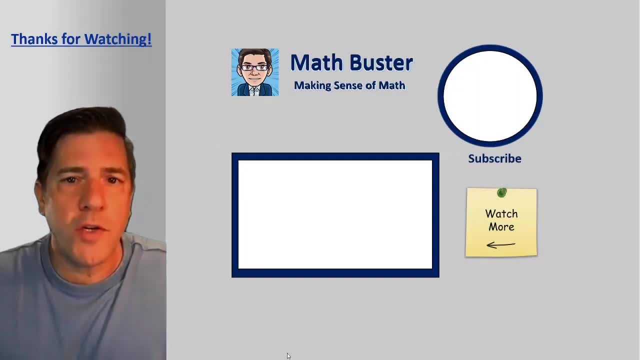 And I've got some more stuff for you to watch right here. Thanks again for watching and please come back soon. 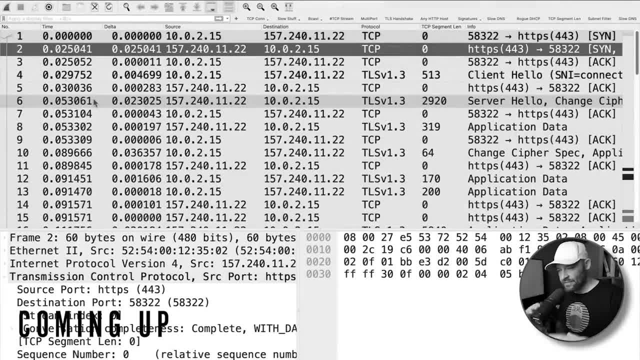 There was a bit of a delay, There was a bit of a lag that was experienced by a user just going out to the internet. Now that user complains, of course it's the network, the network's slow, all the things, This problem. it wasn't super huge, It's not like the person was sitting there. 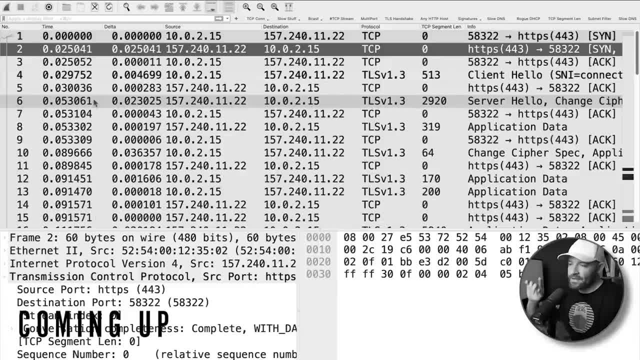 waiting with a spinny wheel for minutes and minutes and minutes. But this example is a snapshot of something that you may see out there in the real world, And I'm going to show you my workflow of how to find it. That's brilliant. You have to do this for yourself. No amount of 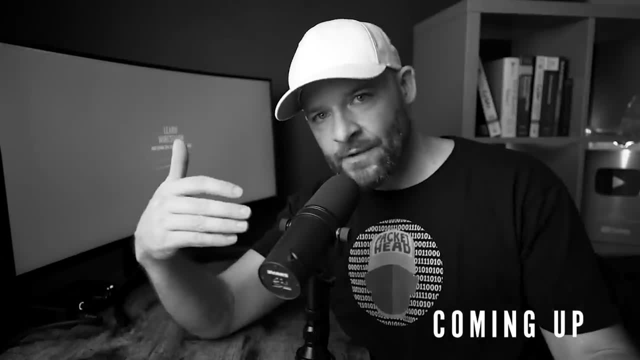 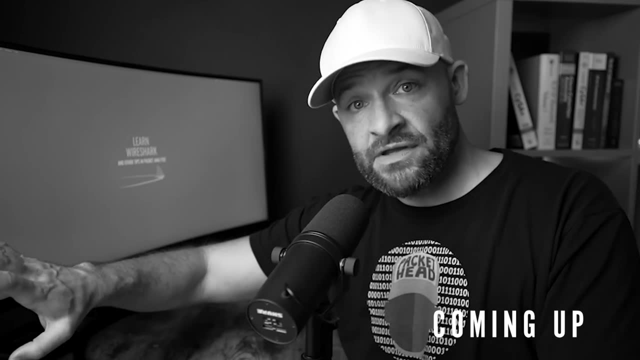 watching these videos out there. everybody, if we can just have a real sidebar, you've got to take Wireshark, open up these captures and dig through them on your own. If you're just watching this video, you're getting something from it, But those of you that downloaded that PCAP and 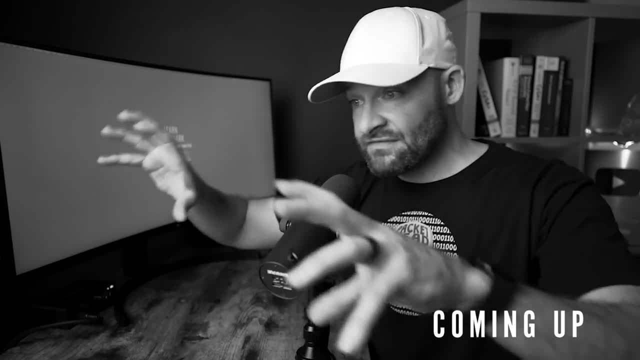 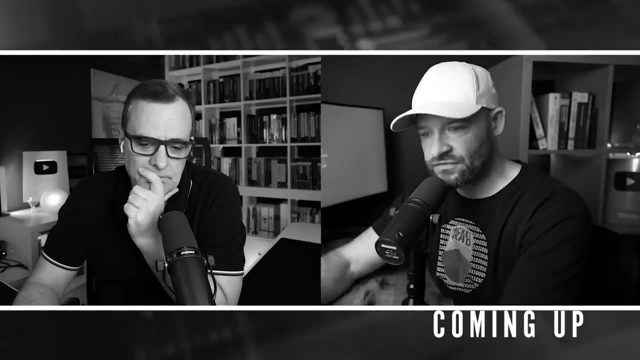 are examining it. if you hit up my channel and do this, if you check out Wireshark and how to configure the screen and these Delta times, if you're doing that, it's going to help you get the most out of it And this is going to become a part of your thought.